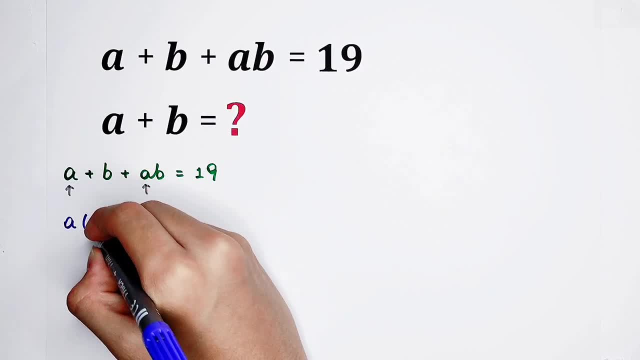 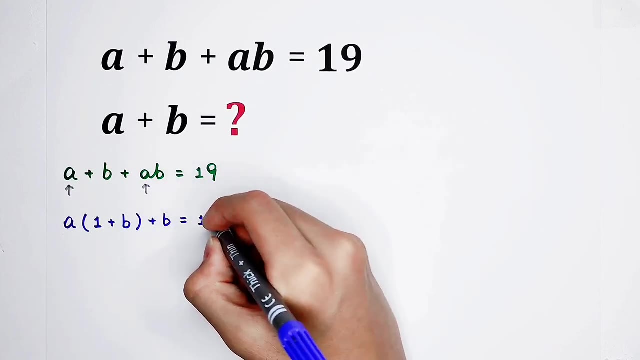 here is a times 1 plus b In the bracket. it is 1 plus b. However, here is a b left In the bracket. I sign 19.. Oh no, it doesn't work. However, I'm gonna say it does work Why. 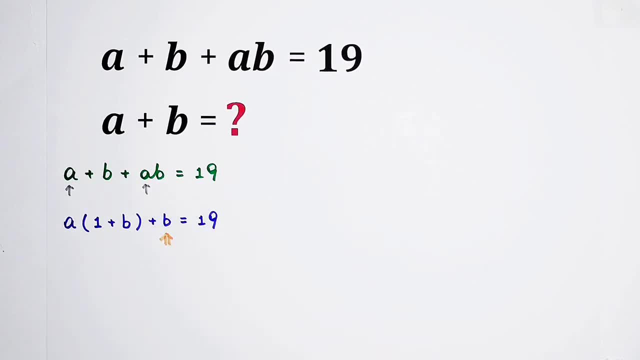 Please have a look at your b, Your cute b. Oh I love it. If you want to factorize it further, we have only one choice. It would be perfect if you could take out a 1 plus b here on the 11 side. 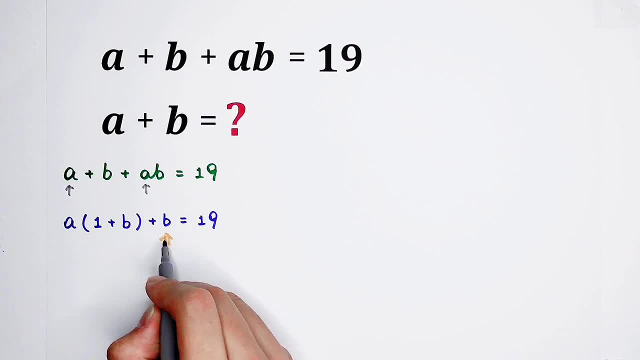 So here is only b. We lack a 1.. What can we do? If we lack a 1, we will create it. We can add 1 on the both end sides. The 11 side will be a times 1 plus b, and then plus b plus 1.. 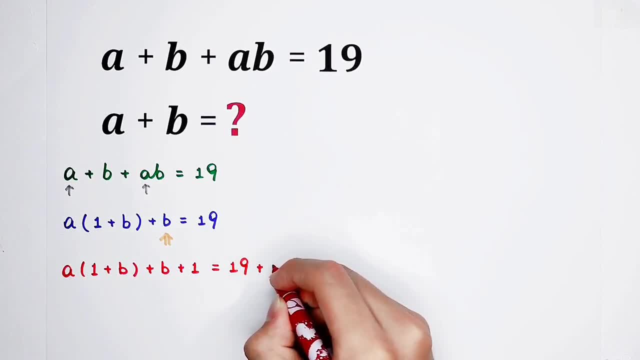 The right-hand side, 19 plus 1.. We've created a- 1.. So here we have b plus 1, 1 plus b. They're actually the same thing, aren't they? So if you take out 1 plus b, here is a, here is 1.. And the right-hand side is 19 plus 1 is 20.. 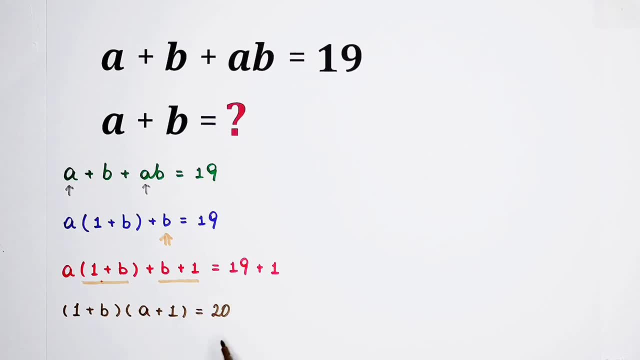 We've done. Although the right-hand side is not 19 anymore, the 11 side has been successfully factorized. The 11 side. to tell the truth, it is so ugly, I don't like it. I don't know if you like it. 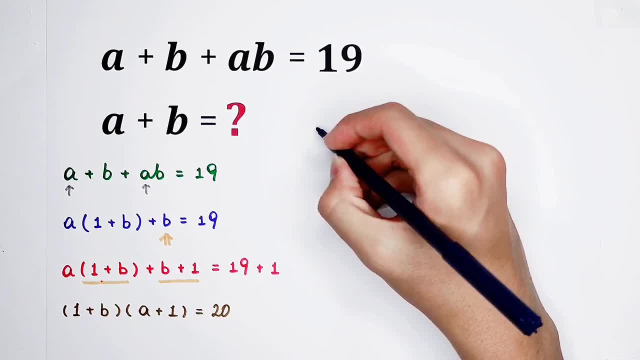 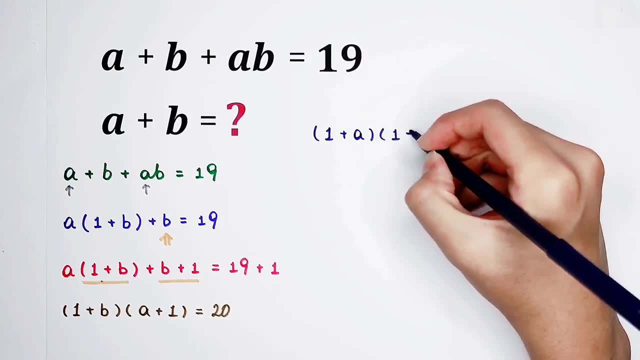 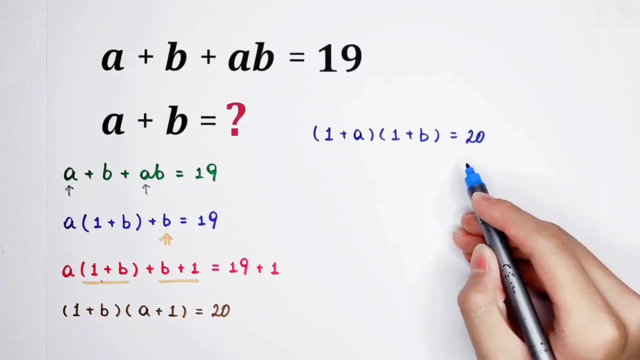 Maybe you like it. So now the 11 side can be written as 1 plus a, then times 1 plus b. The right-hand side is still 19.. The 11 side is still 20.. Now our problem is this: 20. How can we deal with it? 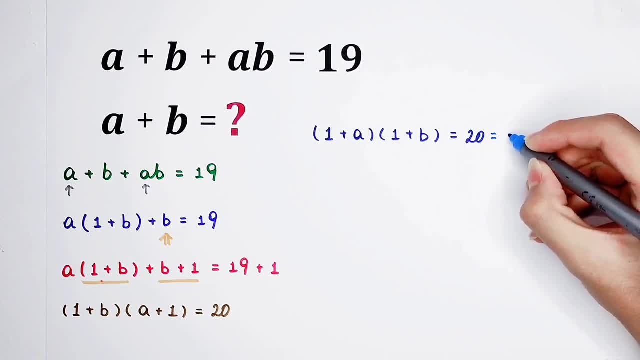 20,. it can be written as 2 times 2 times 5.. So how many possibilities are there? It can be written as 1 times 20.. Also 2 times 10.. 4 times 5.. 20 plus 20 times 1, sorry. 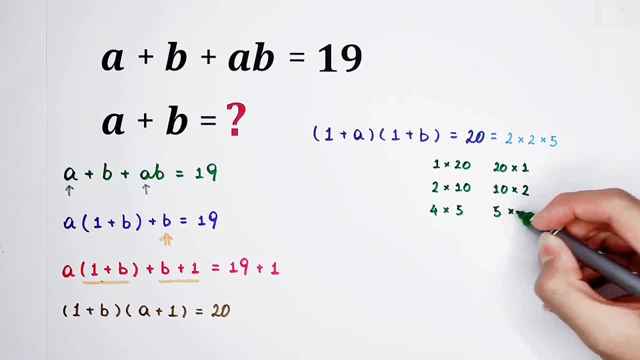 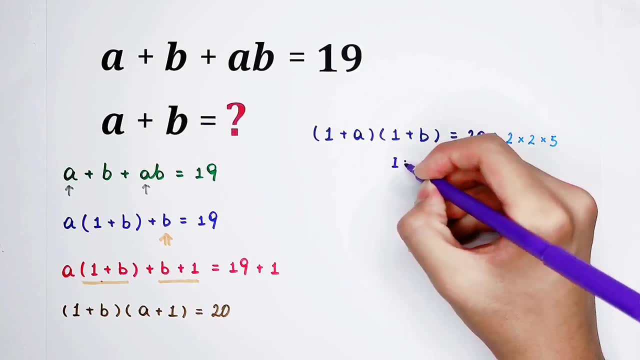 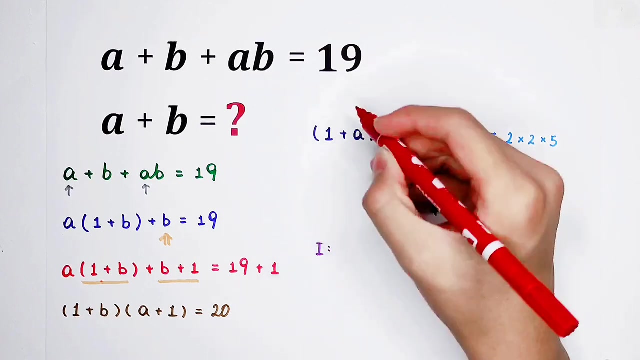 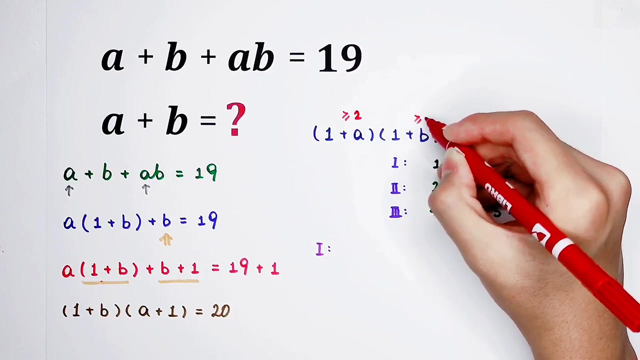 10 times 2 and 5 times 4.. Here I'm going to call them: first group, Here the second, Here the third. For our first group, since a and b are positive integers, so 1 plus a should be greater than or equal to 2, and 1 plus b should also be greater than or equal to 2.. 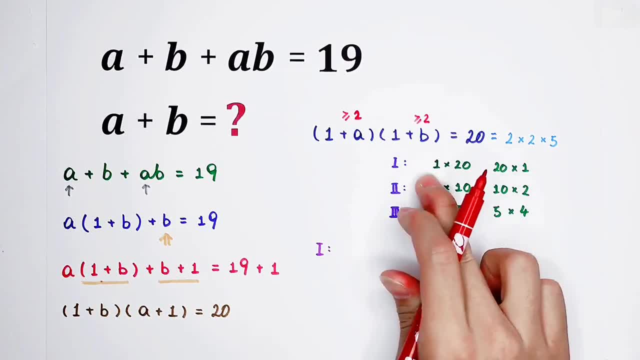 However, in our first case, here is 1.. Here is 1.. So it cannot exist. It doesn't work. It doesn't make sense. Our first group doesn't work, Oh yeah, Then our second group, If we know the value of 1 plus a and 1 plus b. 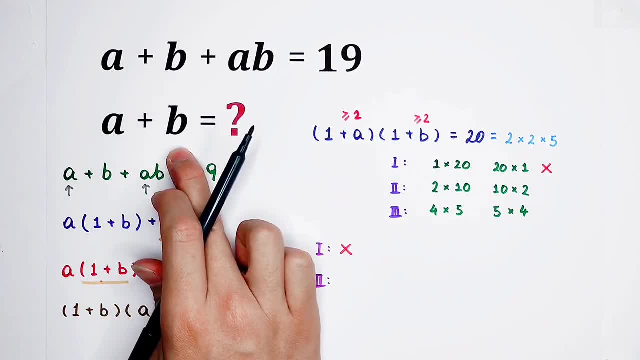 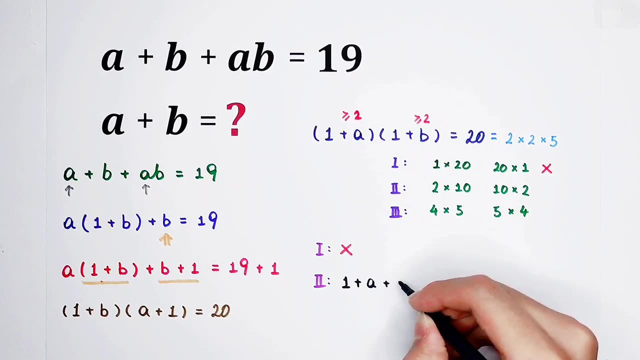 we can then solve the value of a plus b easily. Look For our second group. 1 plus a plus 1 plus b, it is equal to 2 plus 10.. Of course, 2 plus 10 is equal to 10 plus 2.. 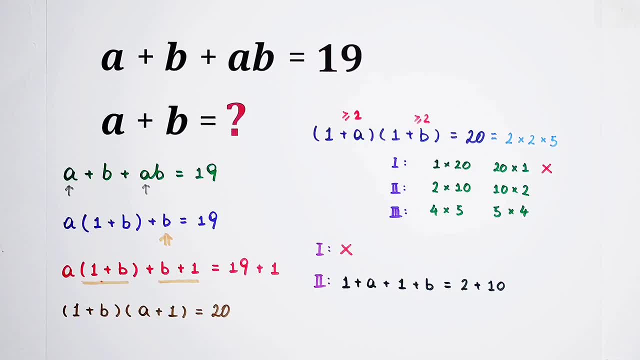 They're actually the same thing. They have the same result In our second group or in our second case. I'm going to say the sum of 1 plus a and 1 plus b is 12.. So the sum of a plus b can be easily solved.